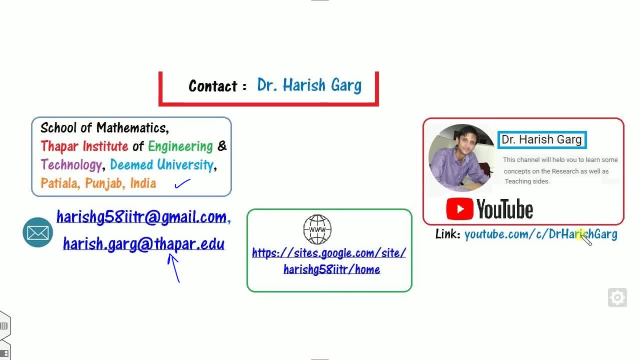 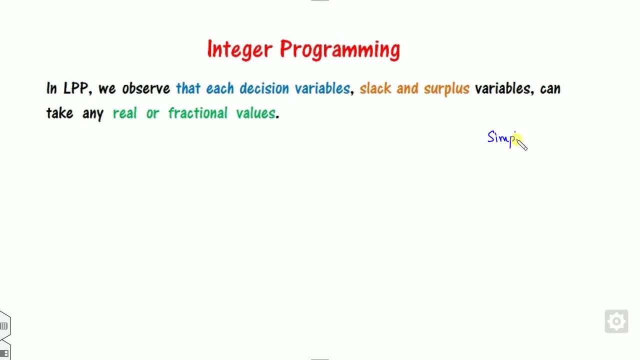 contact me. either of my email ids are there, or else you can simply follow this link for find more updated videos. So, first of all, what we have seen so far is that we have solved several problems with the help of the simplex method, dual simplex method, and many more are there, and 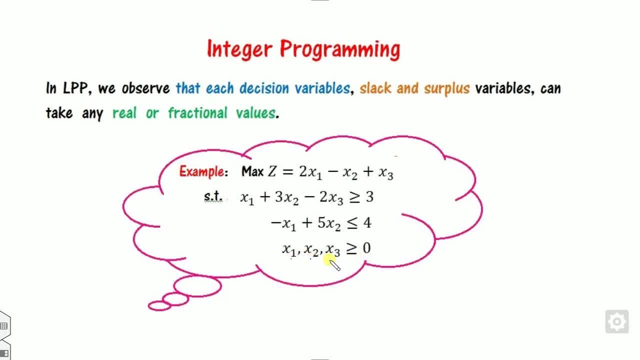 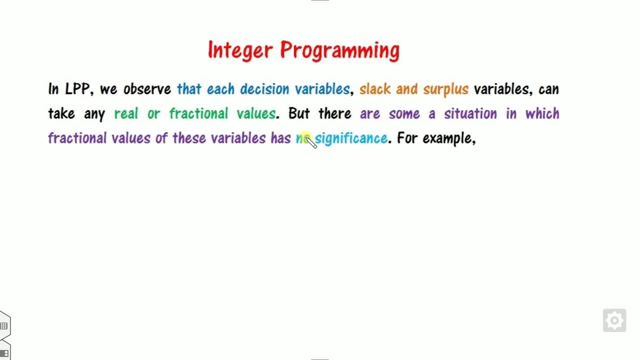 in each of these case we have seen the variables x1, x2, x3 are greater than equal to 0. It means all these variables have either the real numbers, it may consist of the fractional value or it may consist of the integer values are there, But what will happen if we are restricted ourself to be? 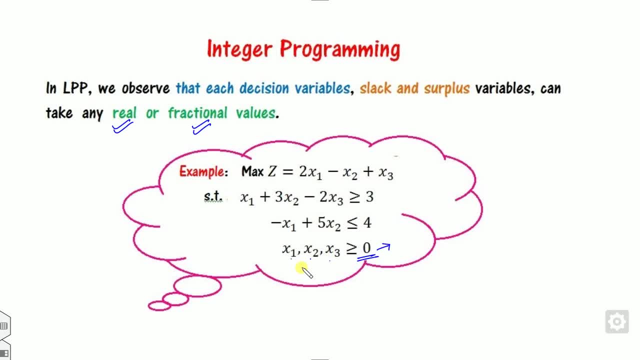 only for the integer programming. It means when we are restricted only for the x1 and x2 are integers, Then in that case whatever we have found, like x1 is 8 by 3, is only for the integer programming. So what we have found is that we have found that x1 is 8 by 3 is only for the integer programming. So what we have found is that if x1 is 6, then we have found x2 is equal to 1 by 10.. That is zero number of used x is bigger than 0. Say if x is amazing. 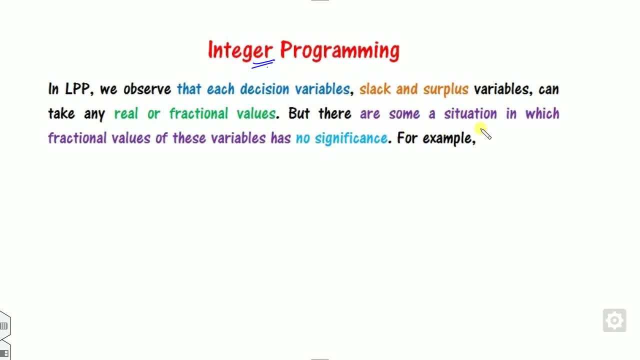 if x is amazing, I cannot add thechange of these marker. x1 and x2 get same if it gets equal to 2.. Same we have. 의 is equal to 1, same, however, x is smaller than x2, when x is big, gears are not used, then % is only used as that number. so when picture is drawing it with 4, and when. if text on one square, it shows where 1 is more than or equal to one square. wait layer stand verses. certainly you should not consider falar this by writing in text. fitness a I met, for example, if I say here a contexto eルstäim in teқs stuff. so for example, 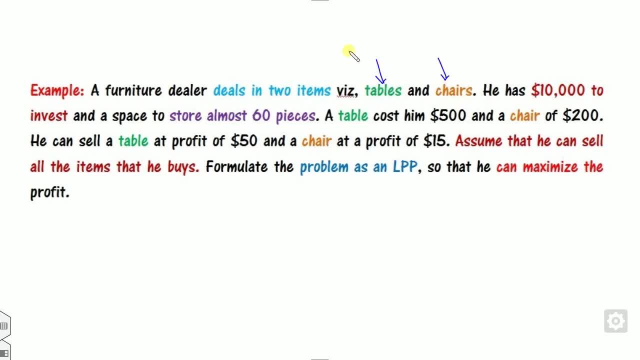 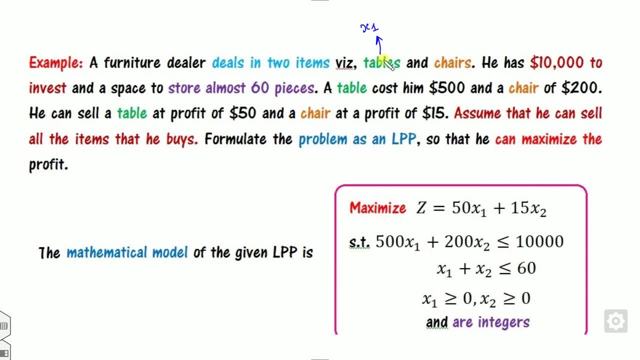 is to deal with that number of the tables and the chairs. so it means you have to construct the, firstly, the model of this, and my task is to find the value of the x1 and x2. x1 is my number of the chairs, tables, and x1- x2 is my number of the tables. chairs and the tables are there. so clearly, sees, 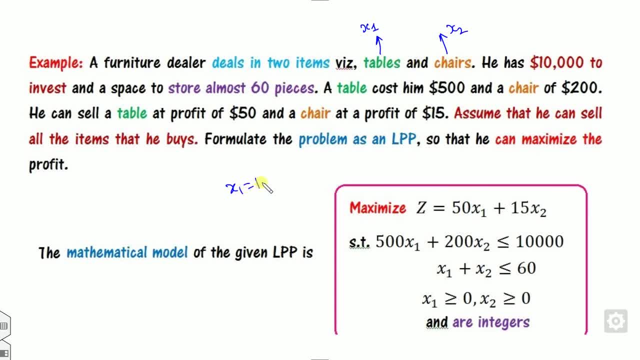 that x1 and x2 are always with the integer numbers. it can't be like 1.5, because a furniture dealer wants to deal with the tables, so they can't deal with the 1.5 tables or they can't deal with the 1.5 chairs. it means we need always be the integer solution. so therefore, if you get 1.5, 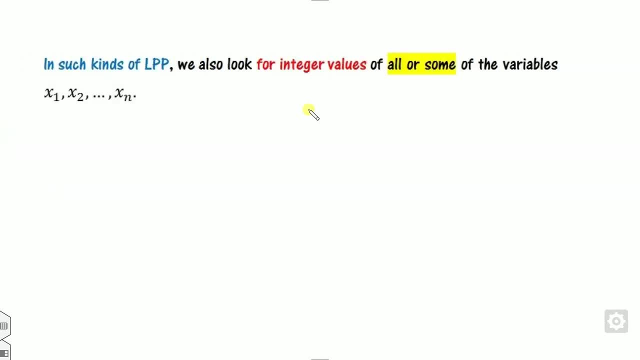 as a solution, then it has the no significance. therefore, for such type of the problem, we always look for the integer values, and integer values or, or some or all of the integer values are there. so what is the definition of the integer programming problem is a problem, a problem. 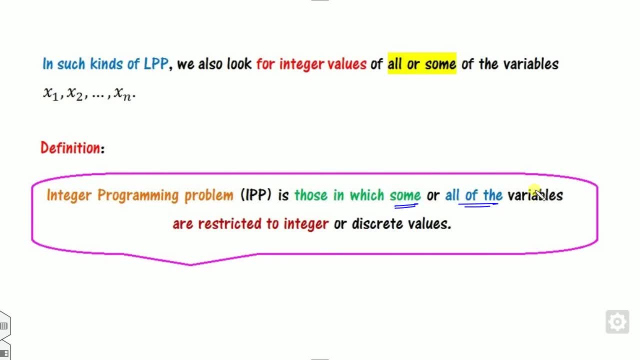 is said to be the integer programming problem, in which some or all of the decision variables- decision variable means whatever you have considered, x1, x2 and so on- are restricted to the integer values or the discrete values. now the question arises here: is that why we need this? 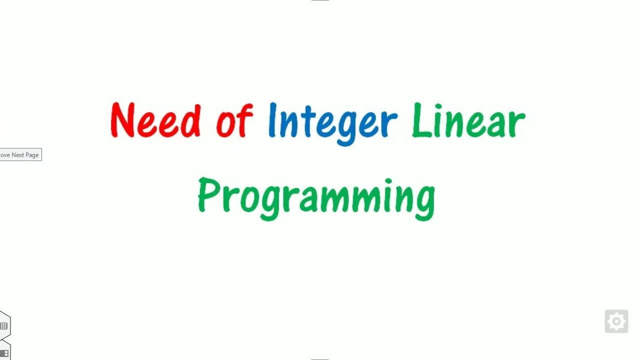 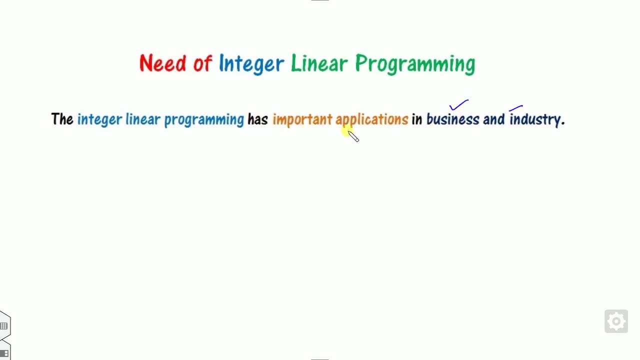 integer programming problem. what is the need of the integer programming problem? so the need is very crucial. why? why? so in most of the business and industry, the integer programming problem is is a huge interest. for example, we can see, for if i say a company wants to assign. 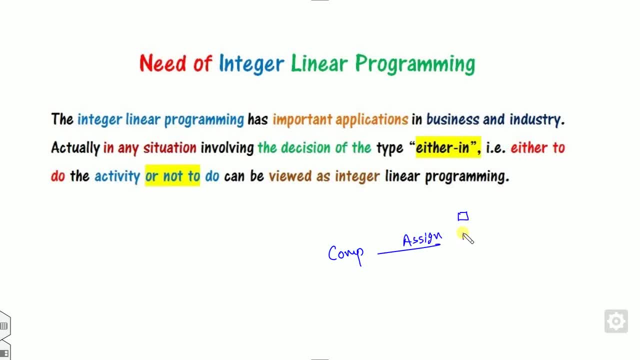 you a number of tables and chairs. so if i say a company wants to assign you a number of tables, a work to a person, so there are the. some persons are there how they can assign a come, how they can assign the work to the persons they can assign either to the this or to this or to this. so 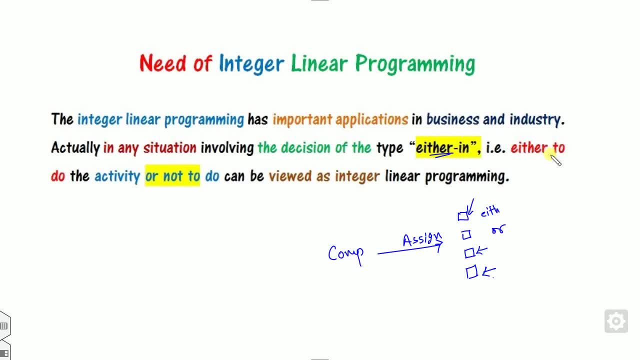 whenever there is a condition of either or or either, in that is, either to do the activity or not to do the activity- we always look for the integer solution. another example which we have seen in our day-to-day life is whenever we want to manufacture the number of tables and chairs. 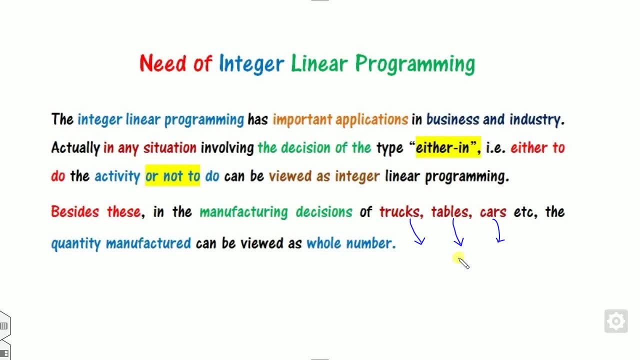 the trucks. when manufacture number of the tables, manufacture the number of the cars. we always look for the integer solution is there because we always want to manufacture the 7.5 cars. is it possible to manufacture 7.5 car? no, we always look for the either 7 or 8 cars will. 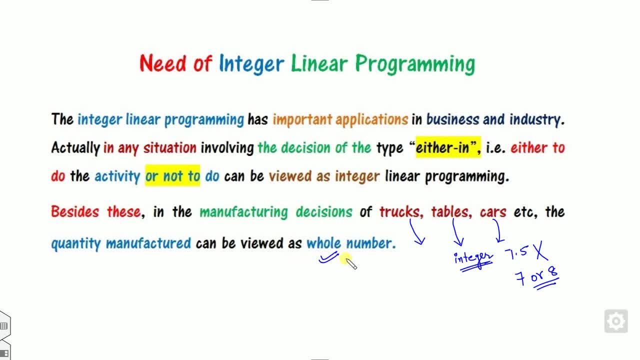 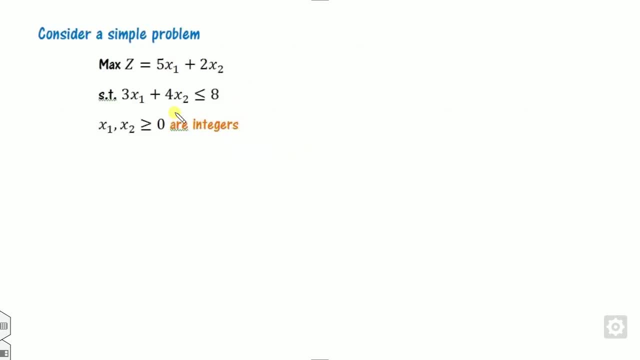 be there and another thing is that. so that's why this always be considered as a whole number is there. so these are the two major important are there and what will happen if we ignore the importance are there, like if you are saying that the engine loose is, this is not working and this. 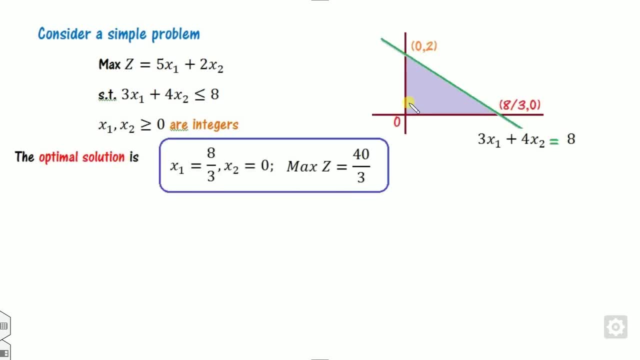 is not running. we also need to be careful that, as you are running with four series, you are at a like, say, what will happen if you solve this problem? So, firstly, I just try to solve this problem with the help of the graphically So we can see. these are there Now. clearly we can see. 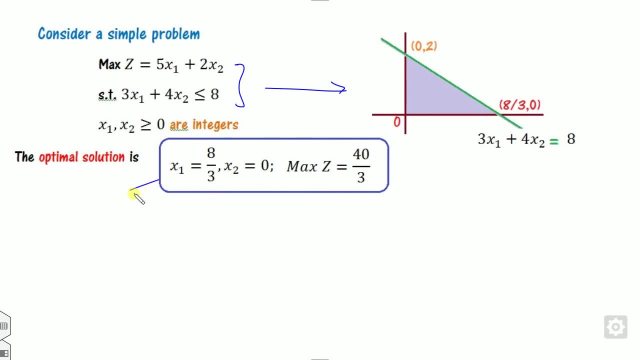 that 8 by 3 is not an integer, So it means this solution is of no use related to this problem. So what is the meaning of that? So this 8 by 3 means that is a 2 point of 6,, 6 and so on. 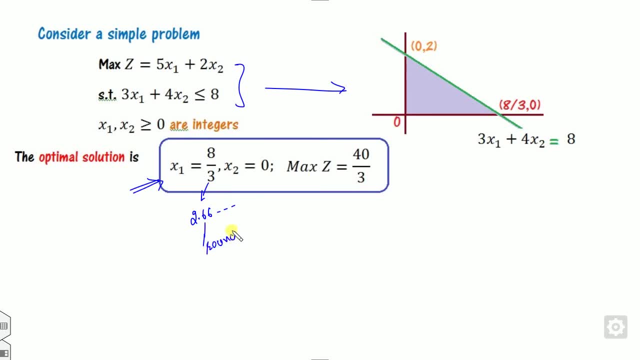 So what will happen if I use, if I round them 2 or we can trunk them? round them means either I can round them 2 or 3.. So what will happen if I round them to be the 3, then the solution will: 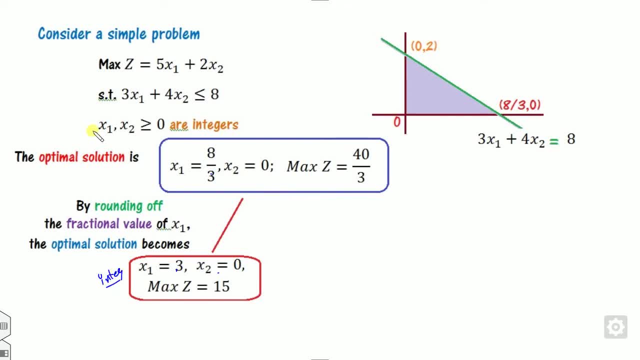 be 3 and 0.. Now it's integer, that's 2, and if you round them to be the 2, that is, you want to trunk them- you will get here. So is this solution is possible? No, Why? Because look at that: 3,0,. 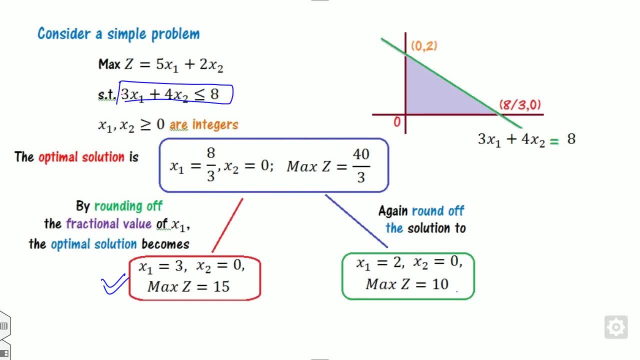 is it satisfied? this one, No 9 plus 0 is, can't be less than 8. So this solution violates this one. So it means this solution is not possible. if you use the rounding, If you want to round off again as a 2,, this is: 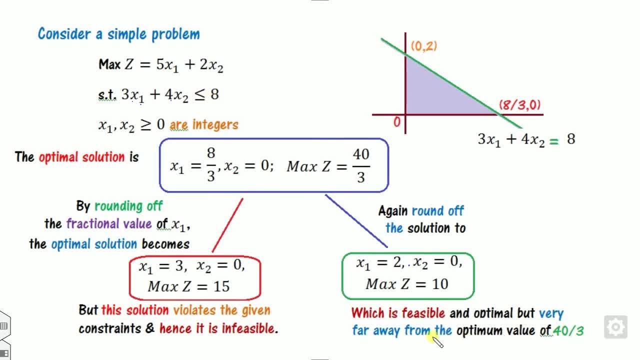 feasible because this satisfy that 6 plus 0, that's 2, but it is very far away from the 40 by 3, that is this solution. So it means in both the cases you get a very: either the infeasible, 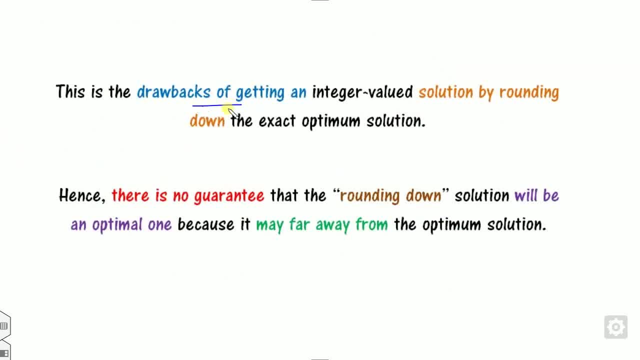 solution or very far away from the optimal solution. Hence this is a drawback, that infeasible solution or very far away from the optimal solution. So it means, in both the cases, integer value solutions by rounding off to the exact value. So you can't that you have to solve. 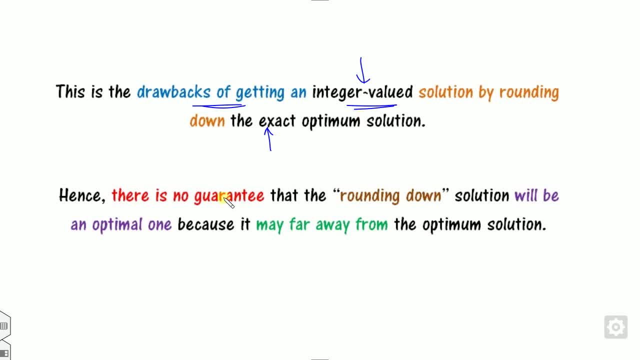 the problem and you can. after that, you can round them. that's a drawback, that? Or you can say that there is no guarantee that the rounding, the solution, will give you an optimal solution. So what are the various types of? so? this is the basic need for the study, the solutions for 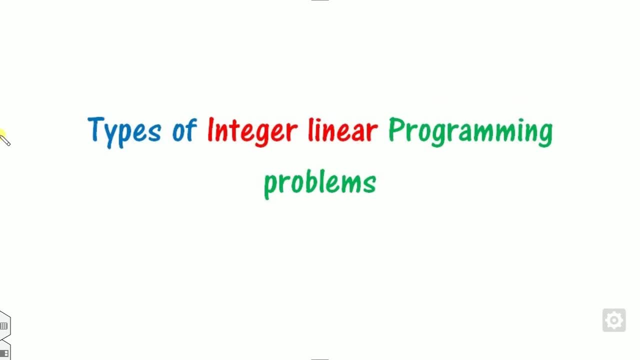 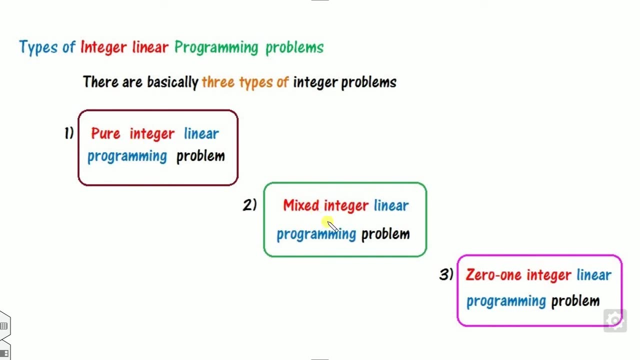 the integer programming problem. So what are the various kinds of the integer programming problem? There are basically three kinds of the integer programming problems. First one is the pure integer. second one is a mixed integer. third one is a 0.1.. So as the name. 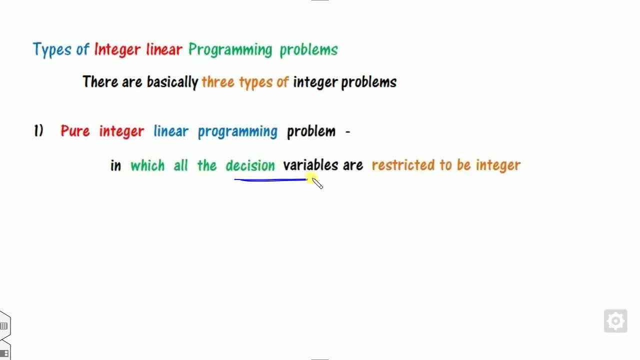 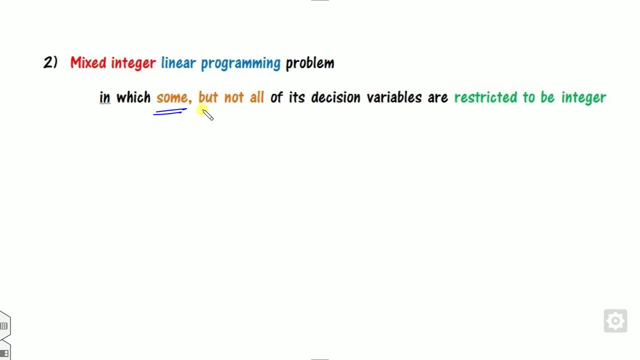 suggests it's a pure integer. So pure integer means in which all the variables are integers, like here: how many variables are there? Three, and in this case all we needs to be the integer. So that's why this is called as the pure. Second type is called the mixed integers, So mixed means. 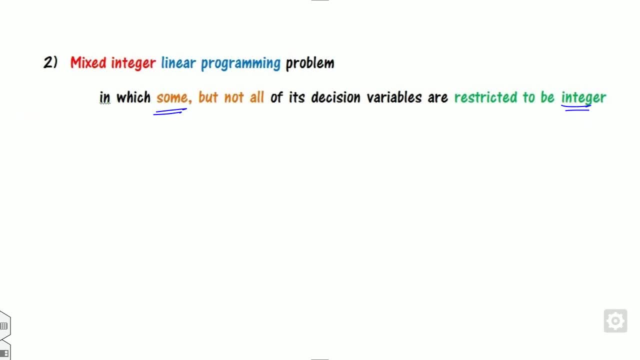 some of the variables are integers, while some may or may not be like here. In this case, we always all we only need. x1 and x2 are the integers, while x3 can be any real number. So that's why this is called as the mixed integers. On the other hand, if some problem is called as the 0-1, let's see: 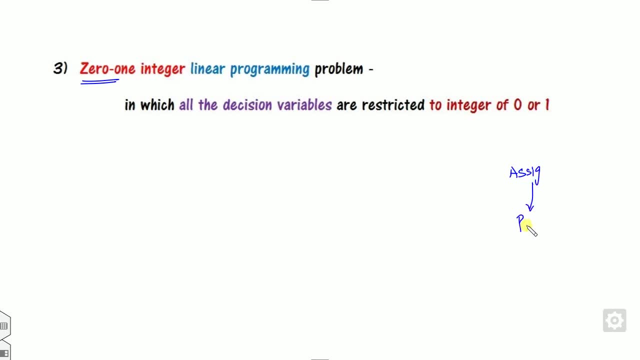 means, if we assign the task to the certain person, then we always perform like assignment: assign the job to the one person only that is working on the 0-1.. So like here, so we will take only either 0 or 1.. Now, these are the three types. are there then? what are the various methods? 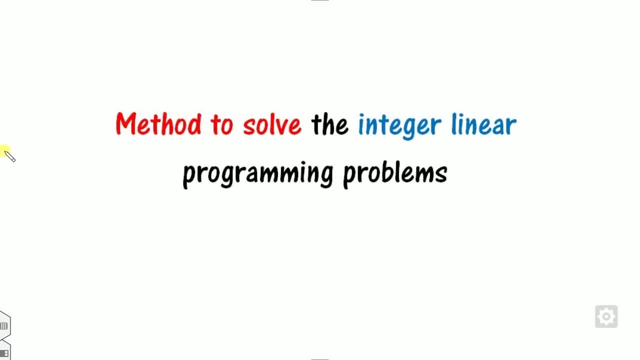 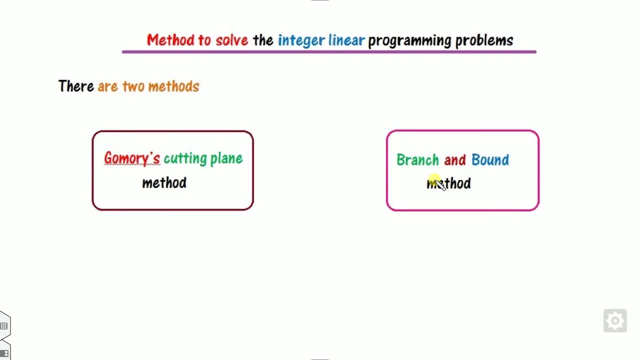 which we can use to solve all these three kinds of the problem. There are basically two methods are there? First one is the Gomory cut plane and second is the branch and bound method, and both are very, very important for solving the integer programming problem. And what is the difference? 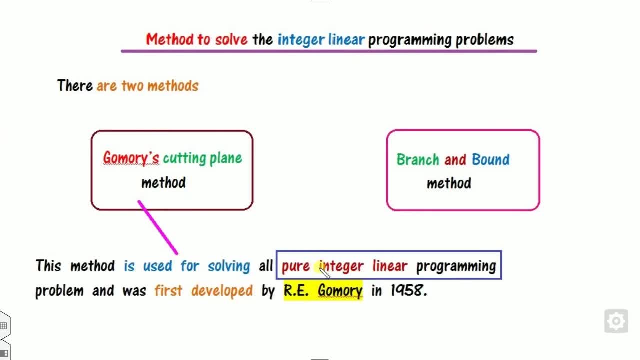 between them is the Gomory cut method is basically used for the pure integer linear programming. pure integer means in which all the variables are all the variables needs to be the integers, and it is firstly developed by RE Gomory in 1958.. That's why this method is called as the 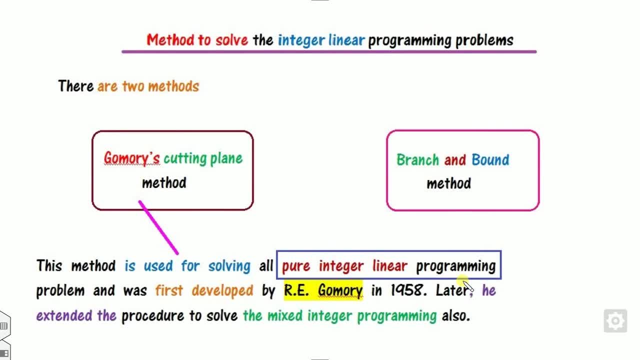 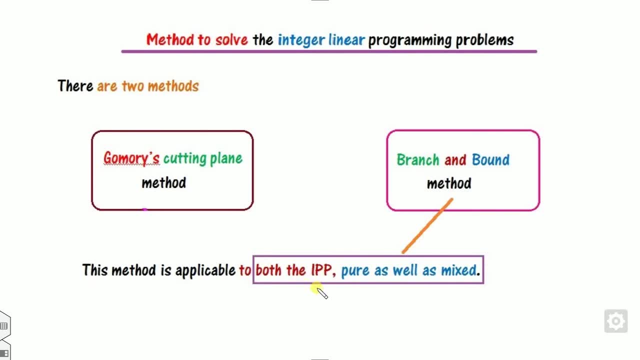 Gomory method and later on after their development. later on he also extended to be the mixed integer programming problem. On the other hand, the branch and bound method is work for both integer programming problem pure as well as the mix, and it is initially developed by 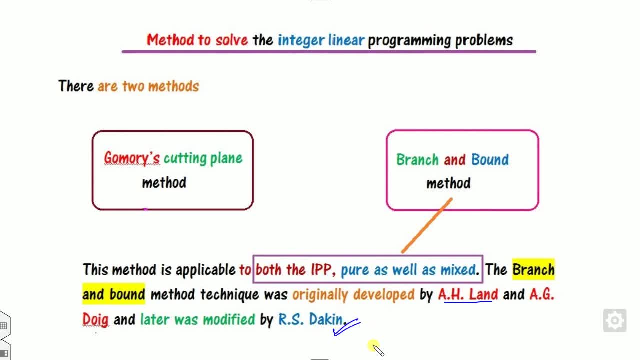 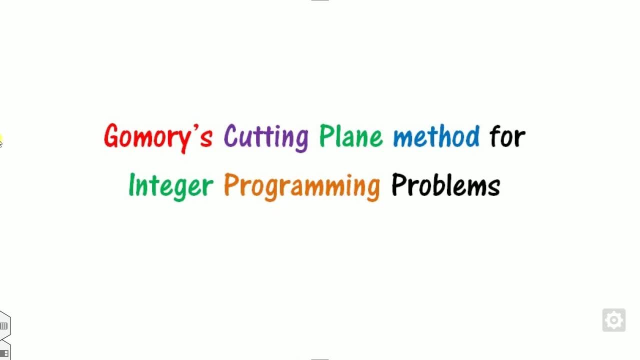 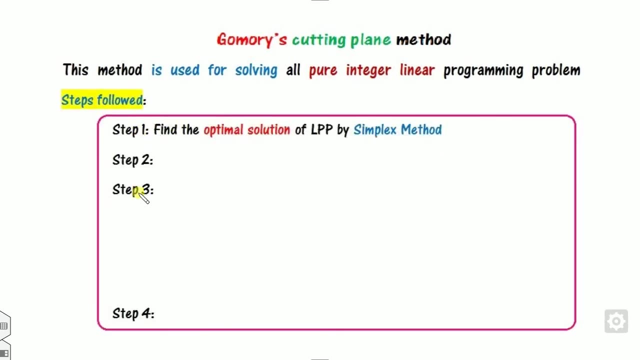 AH Land and AG Dong and later on it is modified by RS Decking. What are the Gomory cut plane method and how it works? we can briefly overview that. So this as we discussed that, it is work for the pure integer methods and it is basically depend upon the four steps. 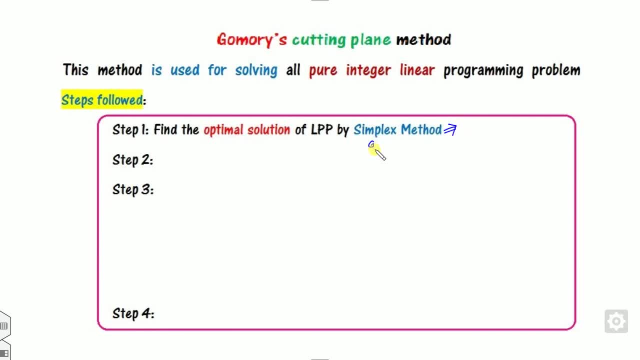 are there. The first step is that you have to solve the problem with the help of the simplex method. You can solve this method with the help of the graphical method, as you wish, or you can solve this problem with the help of dual simplex. Once you will get the here, like say, you will get 8 by 3, x2, as say 4 by 3, x3, as say 7, and 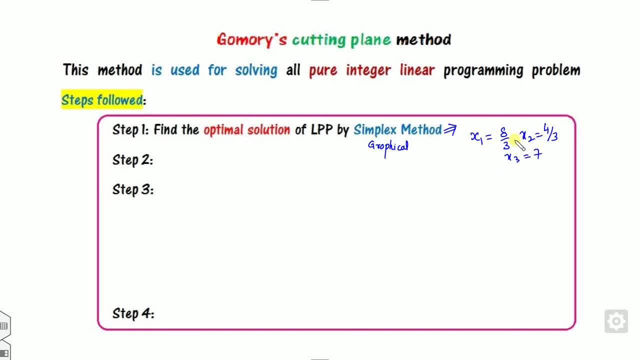 so on, then your second task will be that now, this solution is not the integer, so then you have to follow this step. What you can do is you have. what is the second step is you have to choose the variable which has the largest fractional part. Look at that. what? 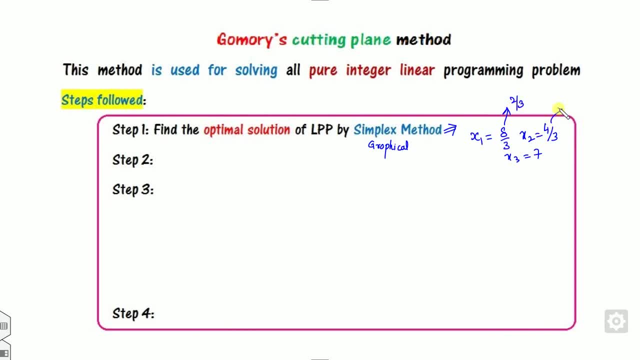 is the fractional part of this is 2 by 3.. What is the fractional part of this will be? I can write as 1 by 3.. Here is 2 plus 2.. 2 by 3.. So what is the largest fractional part is 2 by 3, that is a 0.66.. So I can. 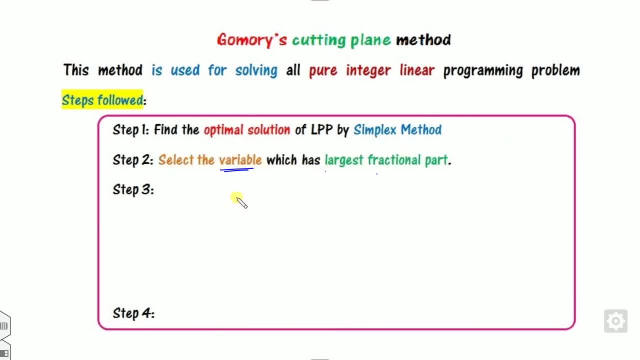 choose the step 2 as the x1.. Once you choose the largest fractional part variable, then we can define the Gumbry constraints like here. What is the meaning of the f1 is that is a fractional component which will always be the positive of the xi row, which, whatever. 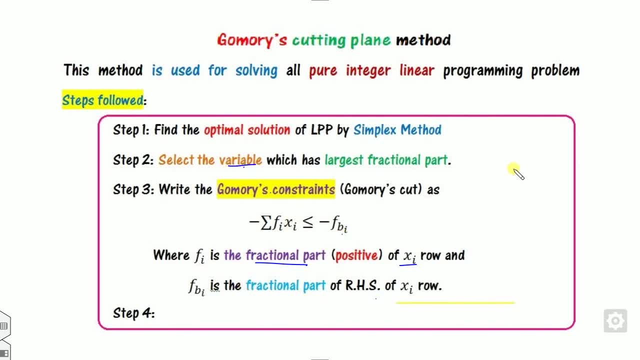 the variable you have chosen, fbi, is the fractional component of this. For example, if you draw the simplex table and if I choose the x1.. These are my say. constraints are here and this is my 1 by 2.. This is minus 1 by 2.. This 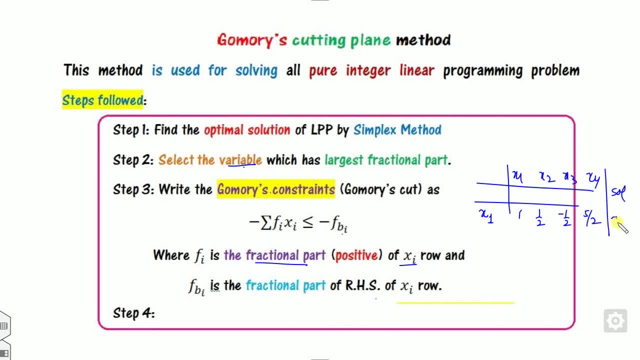 is my 5 by 2.. So, and this is my solution, right hand side is my 7 by 2 or 7 by 3, say So how you can construct them. What is the f1 is? What is the fractional part in the? 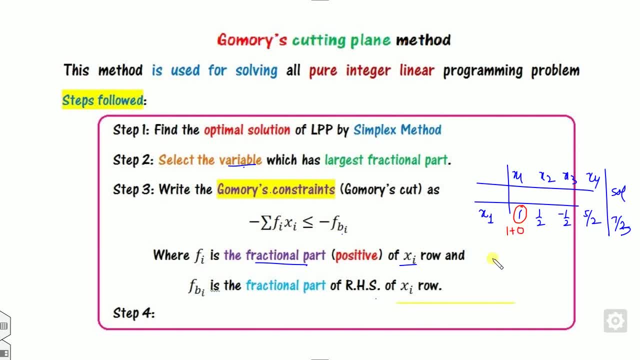 first constraint. So since it is proper integer, so I can write as a 1 plus 0.. So this constant will be 0, x1 minus. Second one is what is the positive fractional part. So this is the x1.. 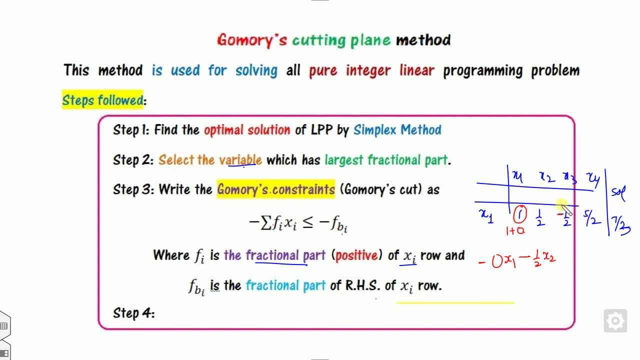 So this fractional part is again half x2.. Now, since this part is negative, so I have to reduce this as minus 1 plus half. Look at fractional part must be the positive. So then this part will be minus half x3.. What is the fractional part of this? 5 can be 5. 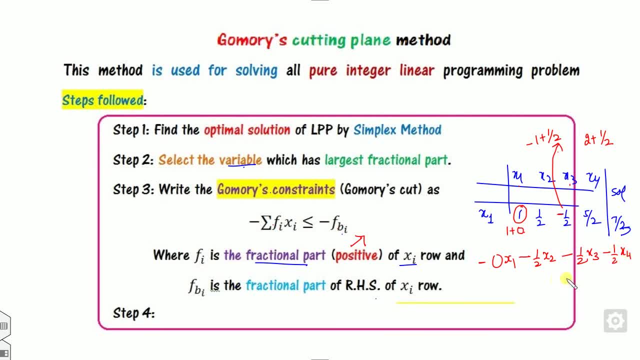 by 2 can be written as 2 plus half. So this is here, which is less than or equal to what is the fractional part of 7 by 3 is. I can write as 2 plus 1 by 3.. So it is here, So. 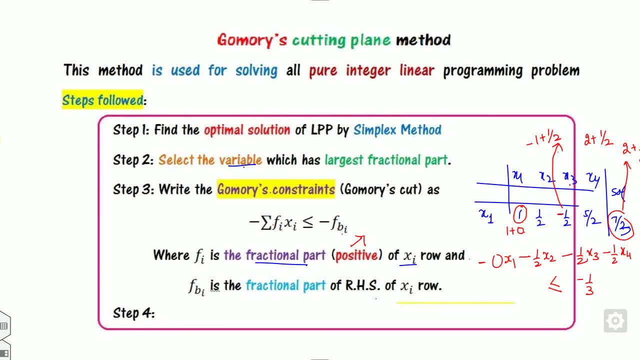 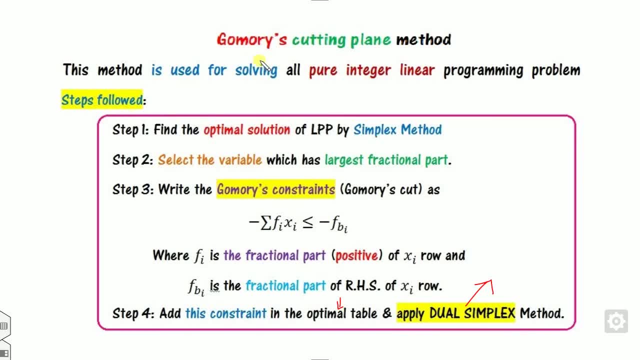 this one has need to be 5 by 2. that isactive. Now if I create another relevant one at x1 plus y is equal to, or equal to 4 by 3, where x 1 is equal to 5 or y is 1 minus 1 or 0. Then 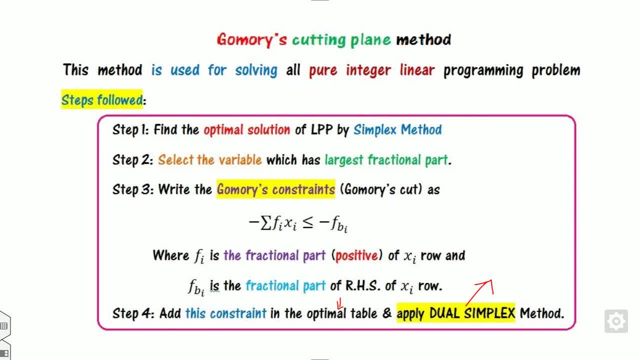 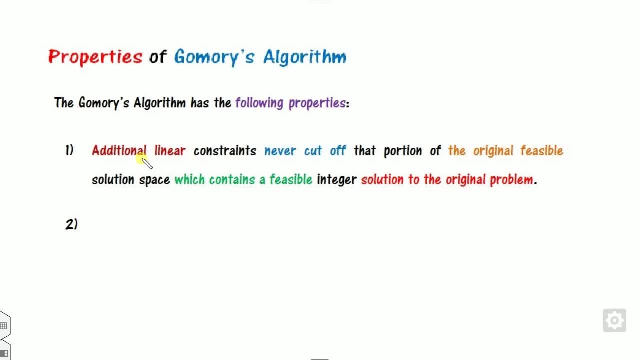 it is a зем restrained. So at x 1 I am writing x1 bound as 0.. Good Steve, 50.. So it means the feasible integer solution will always lies in this constraints. Second advantage is that whenever you are adding the new constraints then it will always 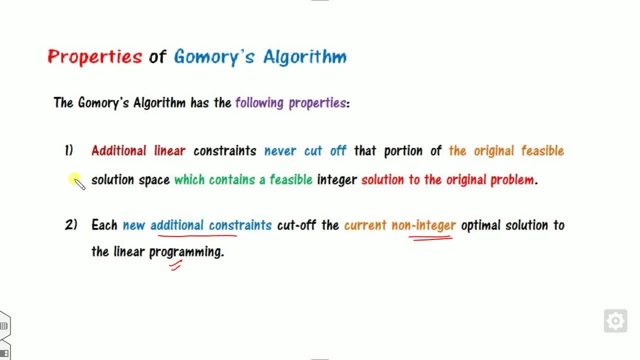 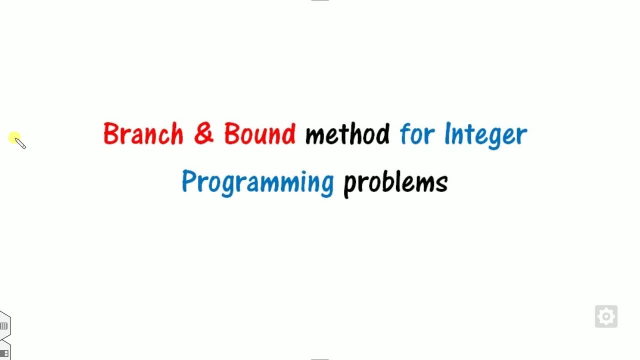 give you the non integer optimal solution to the linear programming. Second method will be the branch and bound method. What is the advantages of the branch and bound method and how it works? So we will see their properties. Firstly, as we discussed that the branch and method is work for the pure as well as the 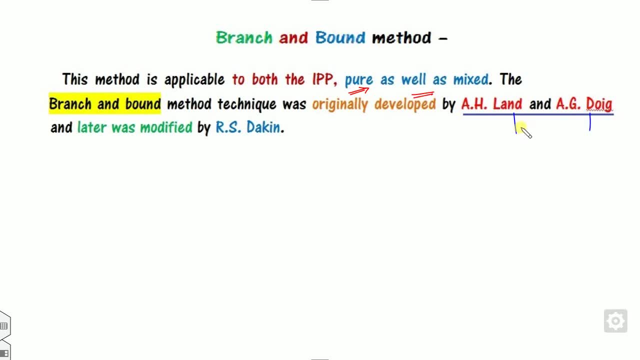 mixed integer both, and it is initially developed by LA Land and AG Gong, later it is developed by RS Deccan. What is the functionality of this method is, In this case, we will firstly find the optimal solution, as in the usual method like graphical 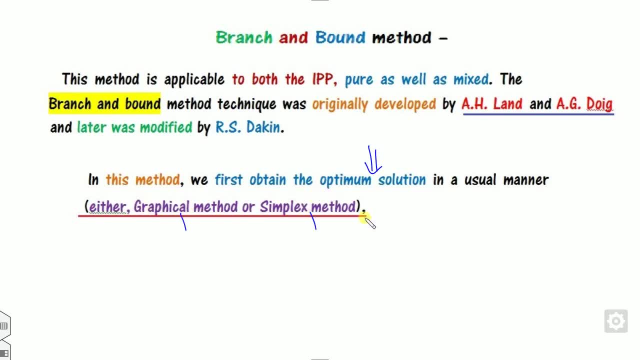 method, simplex method or either of them. Once you are finding the optimal solution, then we will see whether all the solutions are all the variables are integers or not. If it is not, then we will branch and bound. So it means we will divide the feasible area like, say, if my this is my feasible area, 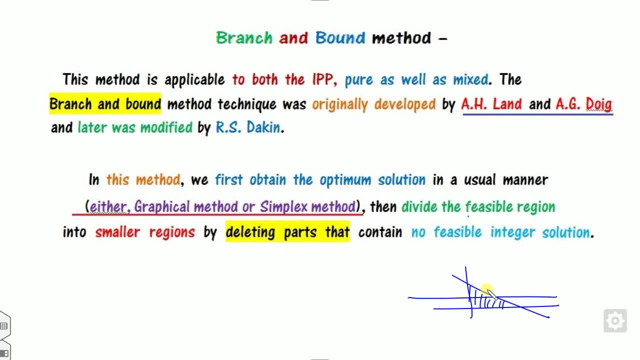 We will divide them- feasible area, either horizontally or vertically. that's the algorithm base. Then we will branch. We will branch them to be the two portion. This is the first feasible area. This is the second feasible area. We divide the feasible area into the smaller region by deleting the parts which contains. 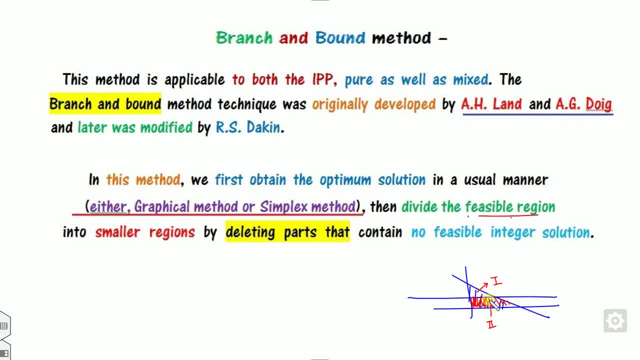 the no feasible solution. So once you are like say, if I say this is the feasible area, now we can find again the optimal solution from here Again we will see. if it does not contain the integer solution, then we can divide again here, and so on. 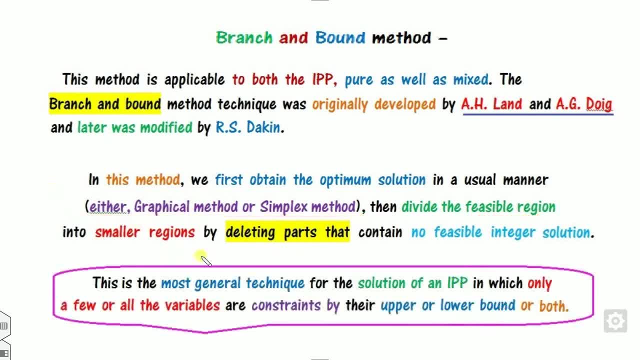 So we can divide the feasible area into the smaller parts and then and so on. So this branch and bound method is the most general technique for finding the integer programming problem. You can also see that the branch and bound method available in the playlist, or else you 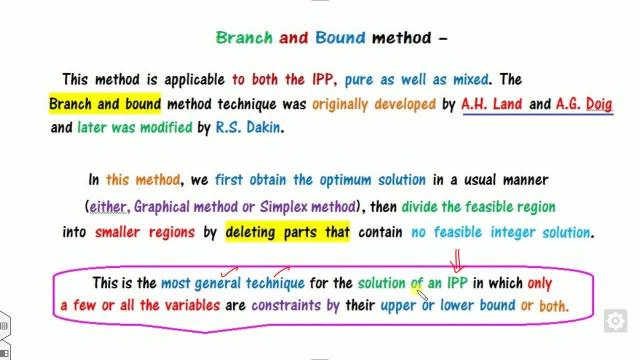 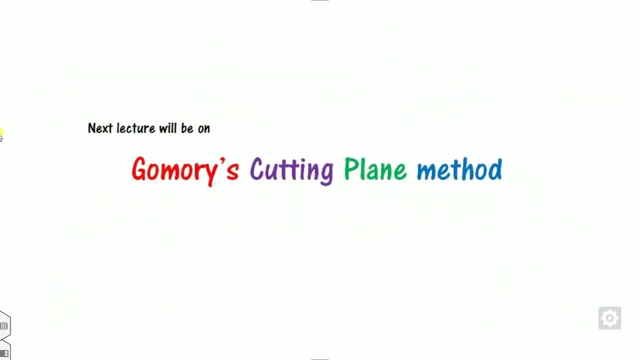 can see in here. the I button link is there. It is one of the most useful technique for solving the integer programming problem. This is not only the few, but all the variables are the constants as a lower and the upper bound. So these are the simple functionality of the two methods are there. 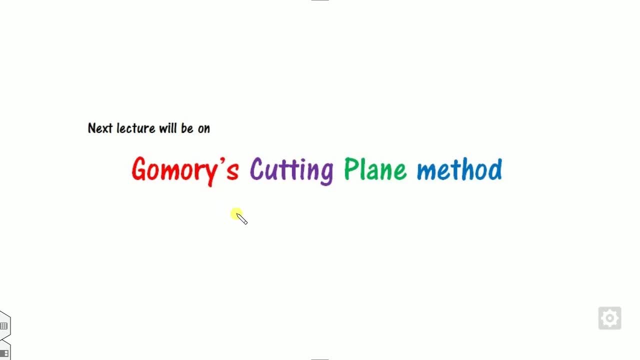 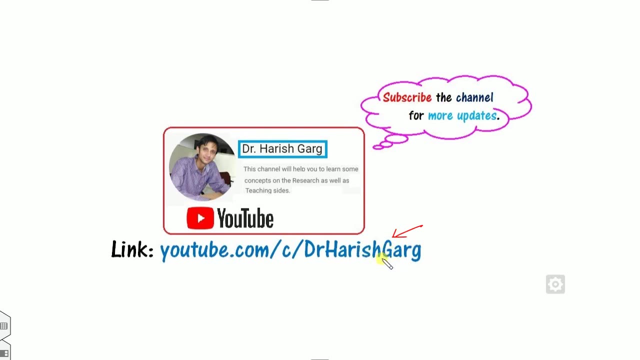 We will see how this Gomery-Kurt methods will work with the help of the several examples in our next class. Till then, you can find these other videos in this YouTube channel link. You can find it and share this video to the other.